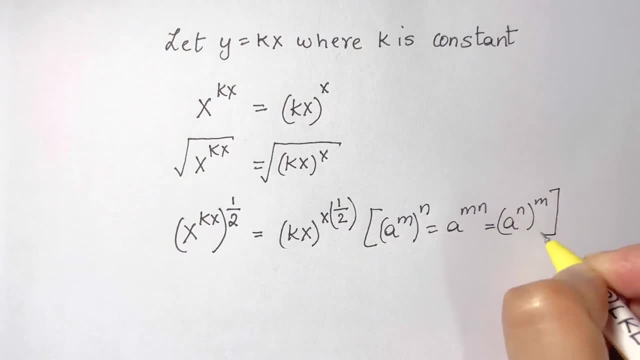 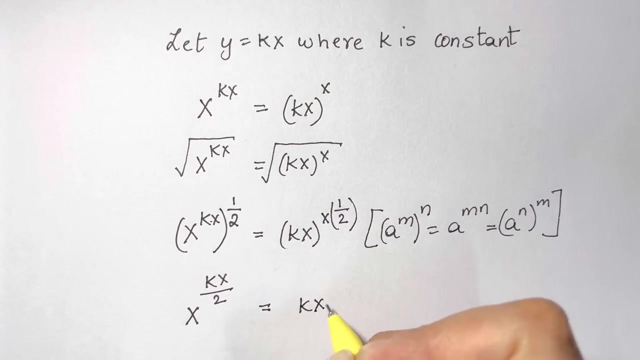 a to the power of n. whole to the power of m. You can even write it like that. So we are going to apply this Here. we have x to the power of kx over 2. Which is equal to kx over x over 2.. We just multiplied the powers. 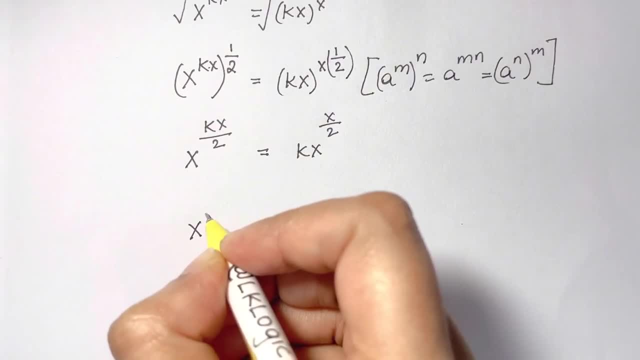 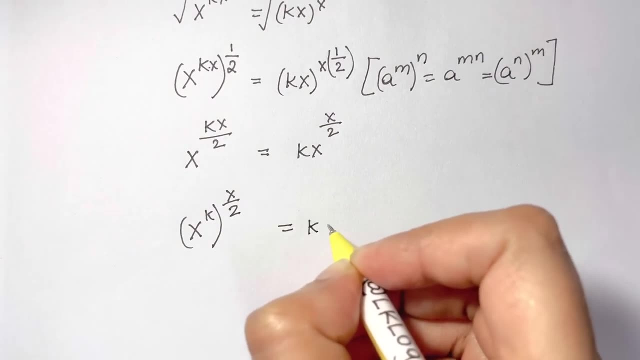 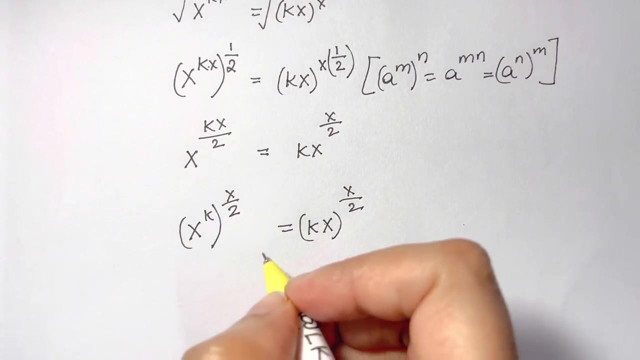 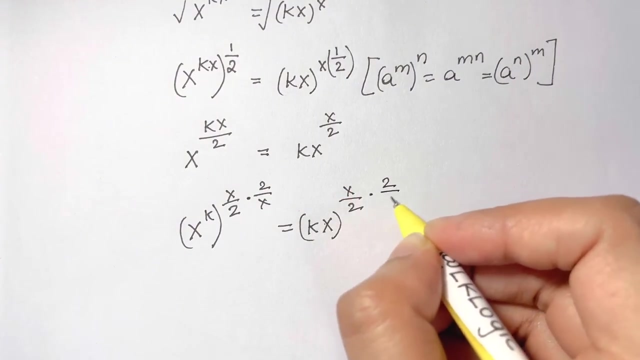 Now what do we get? x to the power of k. I can write it like this: Whole to the power of x over 2.. And here also x to the power of kx, Whole to the power of. I only have x over 2 here. So now, when I want to eliminate this power, I will just multiply both sides by 2 over x, Times 2 over x, So I can cancel it out: 2,, 2,, x, x. And here also the same thing. 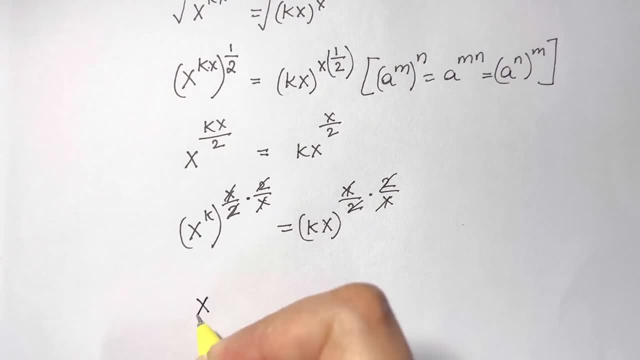 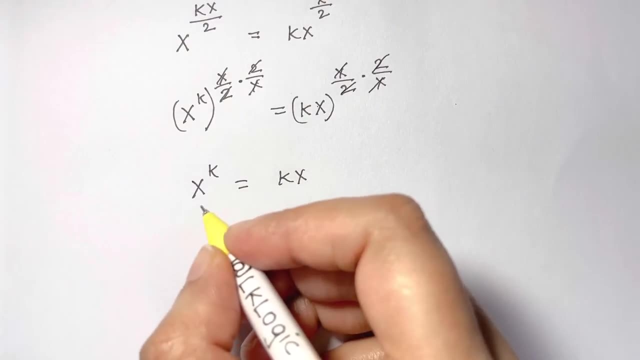 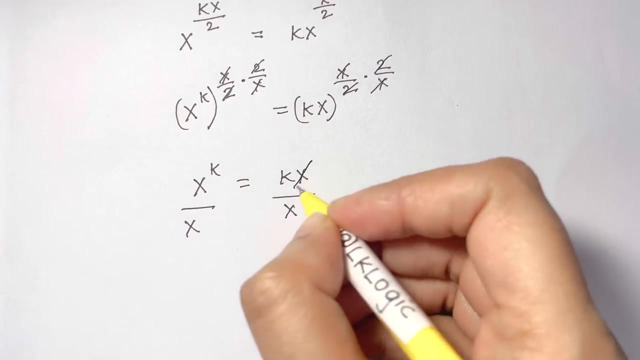 Then we are left with x to the power of k is equal to kx. Now we have an x here. Let's find out x in terms of k. So I need to eliminate this x from here. So divide both sides by x To eliminate this x Here. I am going to apply this law. 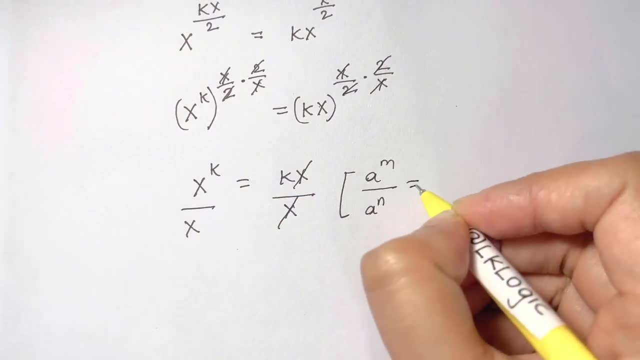 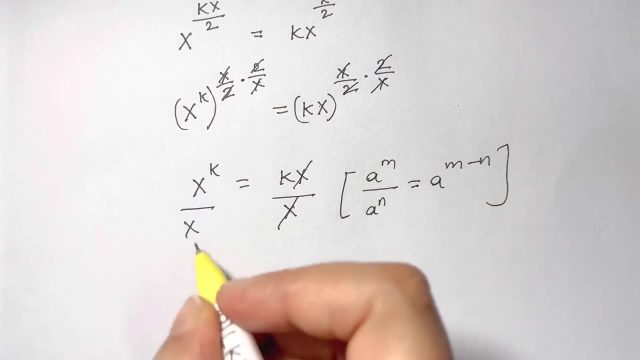 a to the power of m over a to the power of n is equal to a to the power of m minus n. Whenever you have same base and there is division between them, you subtract the powers. So here I have same bases. There is division between them. Let me subtract the powers. The power here is 1.. 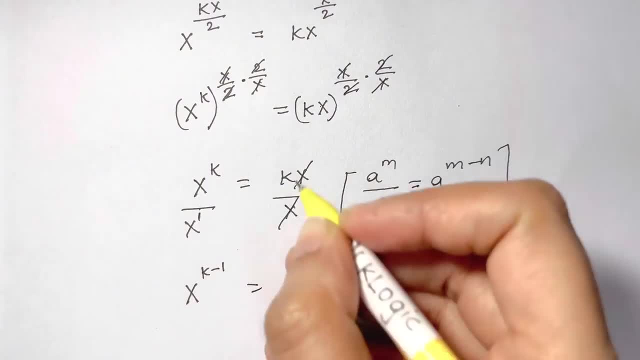 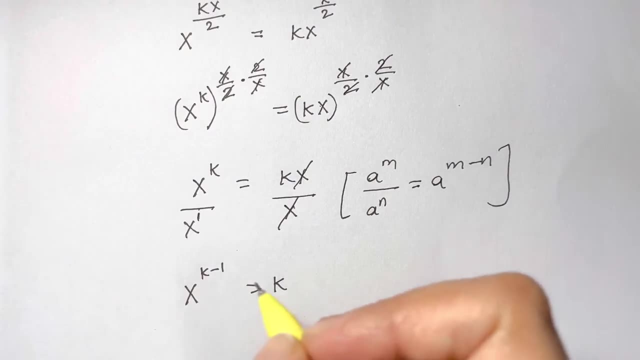 So we have x to the power of k. This is equal to k minus 1 is equal to k. Now what I am going to do is just multiply both sides. This is k minus 1.. So now what I am going to do is just multiply both sides by 1 over k minus 1.. 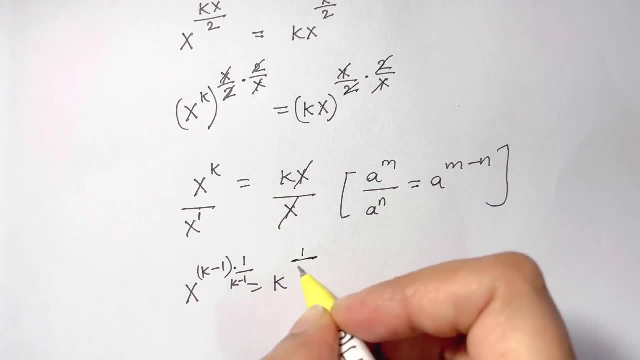 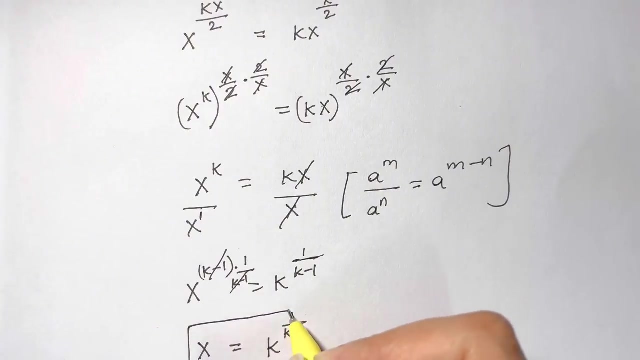 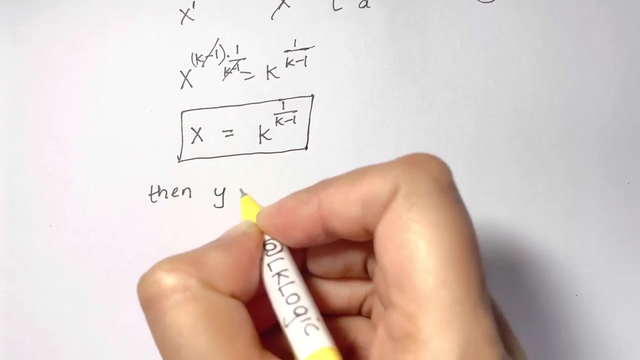 And here also. then we have to put 1 over k minus 1.. So here k minus 1, k minus 1 gets cancelled. So you are left with x is equal to k, to the power of 1.. k minus 1. so we got the value of x in terms of k. then y is equal to kx, so y is equal to. we've got. 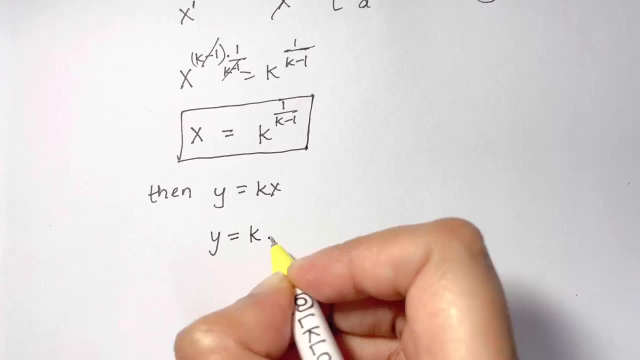 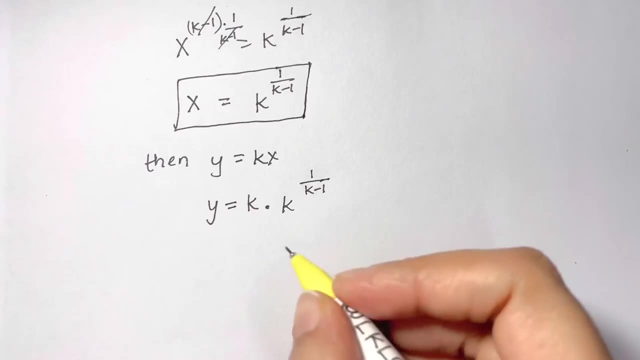 what is x? let's substitute k times x is k to the power of 1 over k minus 1, so k to the power of 1 over k minus 1. we have same base and there's multiplication between them, so we have to add the powers, so y is equal to k to the power of 1 plus 1 over k minus 1, as this is a fraction. 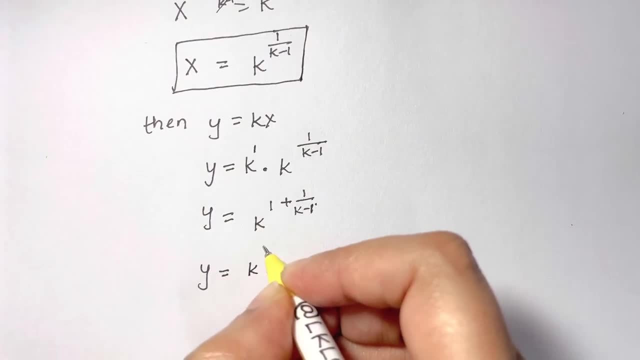 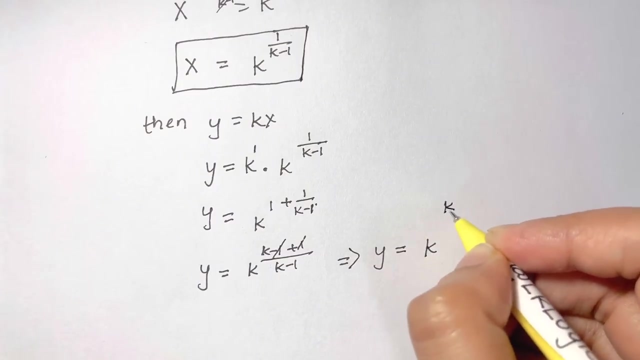 y is equal to k, to the power of k minus 1 plus 1 over k minus 1. when you take the else, and minus 1 plus 1 gets cancelled. so you're just left with: y is equal to k, to the power of k over k minus 1. so this is the value of y which you get. 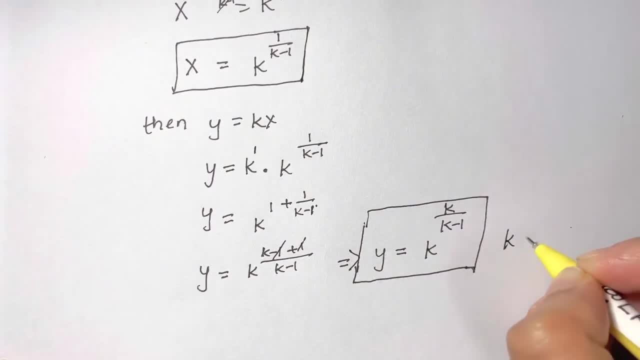 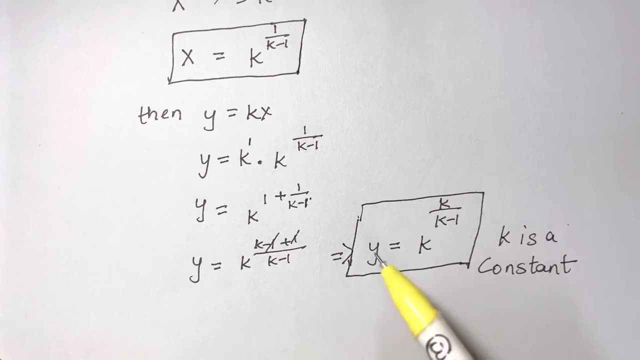 and k. here is a constant. so we have x and y in terms of k, so we can substitute a value for k. example, if we take a x and y in terms of k, so we can substitute a value for k, so we can substitute a value for k. 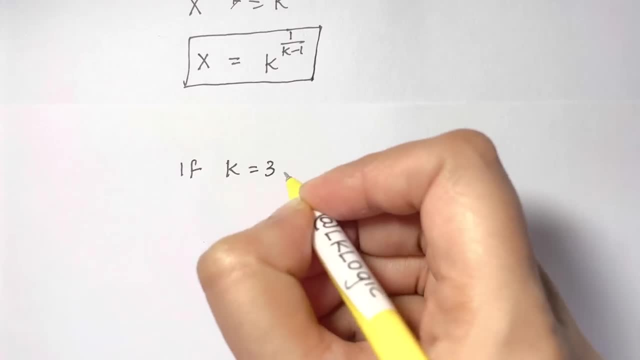 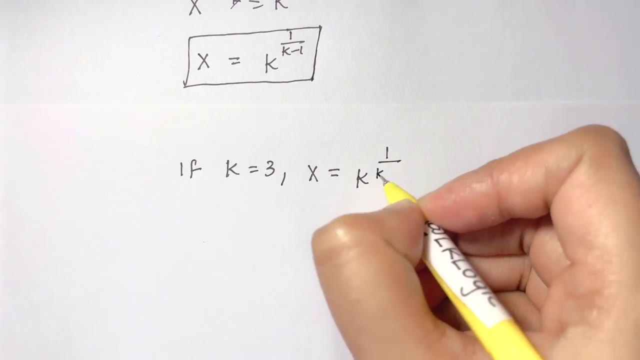 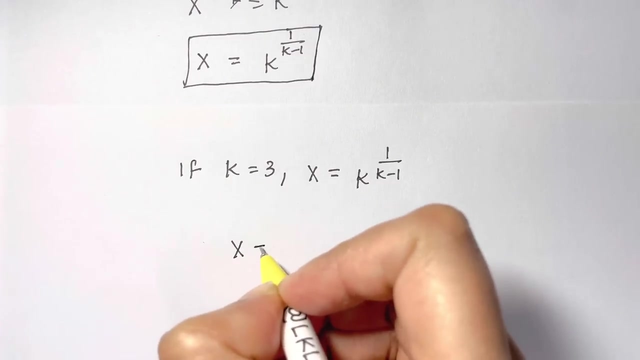 if k is equal to 3, we know what is x. x is equal to k to the power of 1 over k minus 1, so we're going to substitute 3 in place of this. so we have: x is equal to 3 to the power of 1 over 3 minus 1. 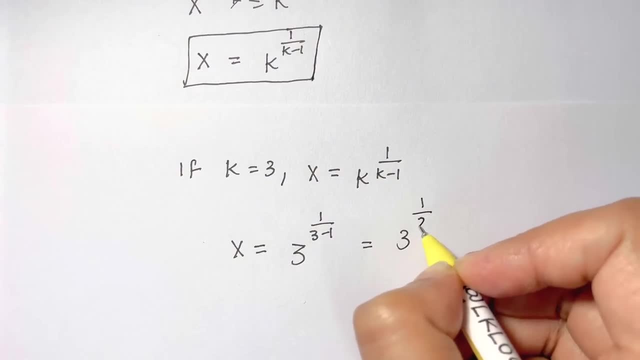 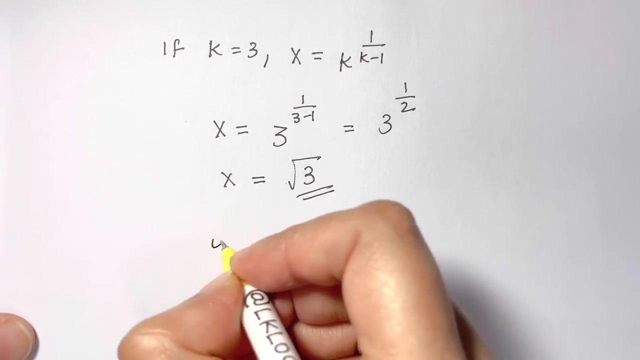 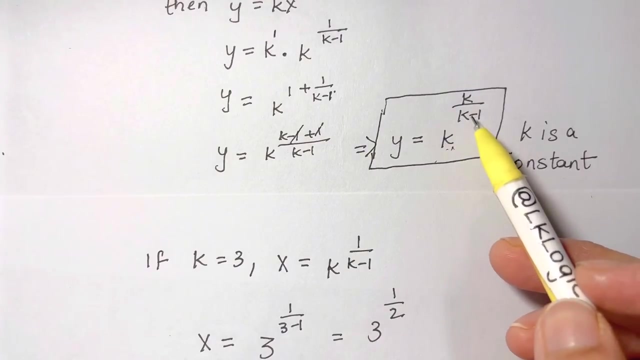 which is equal to 3 to the power of 1 over 2. so x is equal to square root of 3. now what about Y? let's find out why. Y is equal to what we got Y from here as K to the power of K over K minus 1. so we need to write that Y is. 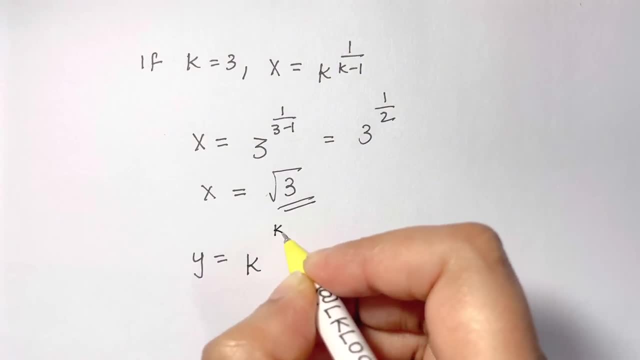 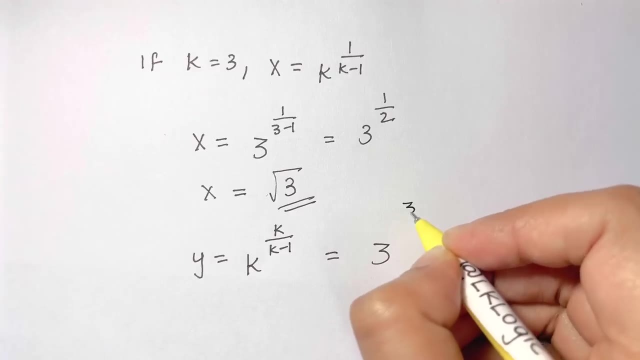 equal to K to the power of K over K minus 1. let's substitute 3 in that, so we get 3 to the power of 3 over 3 minus 1, which is equal to 3 to the power of 3 over 2, and the first is the power and this is the root. so we have to convert it. 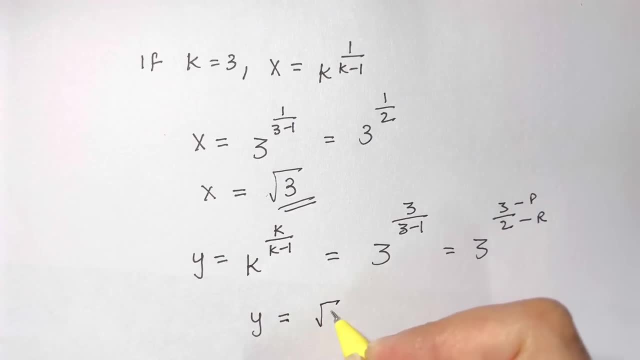 back. so Y is equal to square root of 3, whole to the power of 3. so this is the value of Y. now, if we want to check the X&Y values, X is root 3, wise square root of 3, whole to the power of 3. 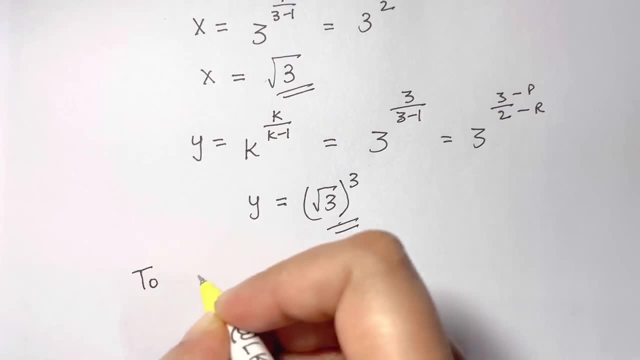 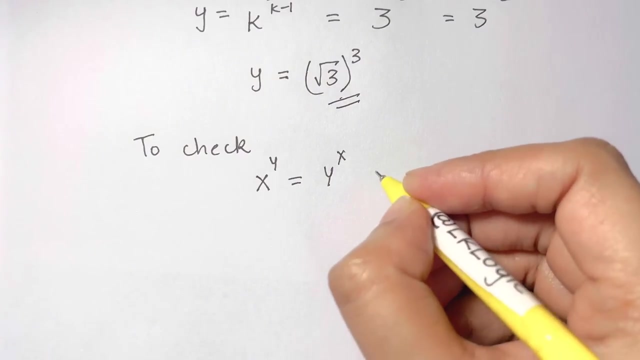 to the power of 3. so if you want to check and the values are right or not, we want to substitute in the main equation: x to the power of y is equal to y to the power of x. so what do we get here? what is a? what is the value of x and y? x is equal to root 3. as we've got here, x is equal to root 3. 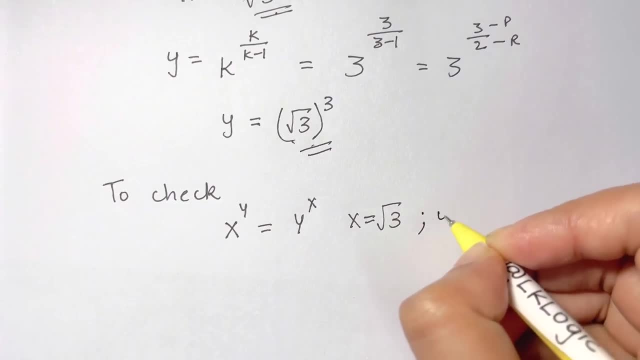 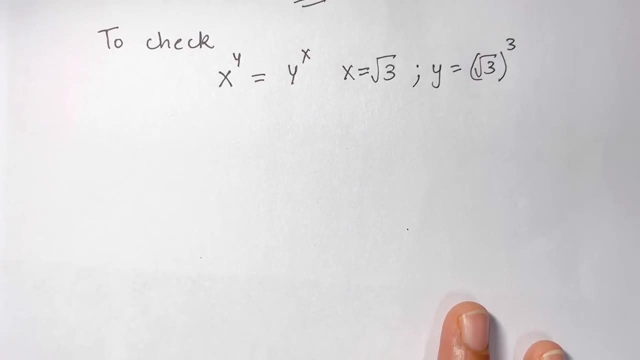 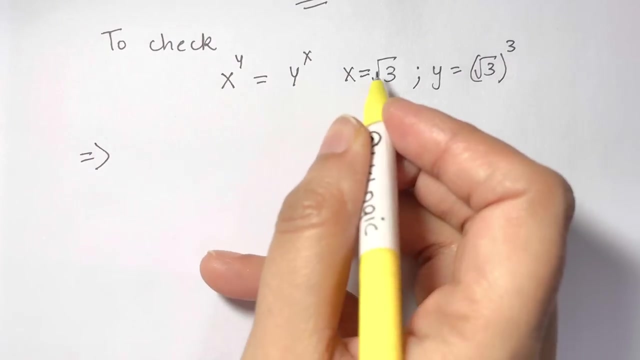 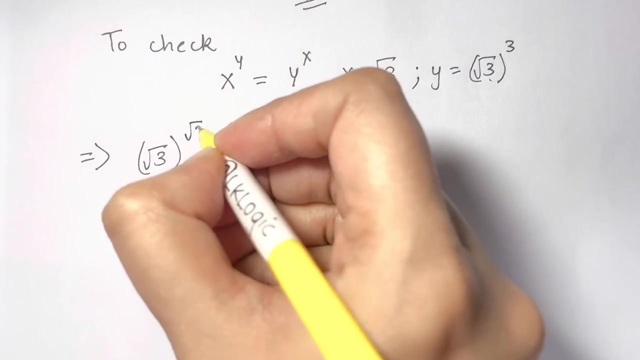 and y is equal to square root of 3, whole to the power of 3. so we're going to substitute that to verify your answer. so what do we get? so we're going to put x as root 3, root 3 whole to the power of y. is root 3 root 3 whole to the power of 3, which is equal to now what is y root 3? 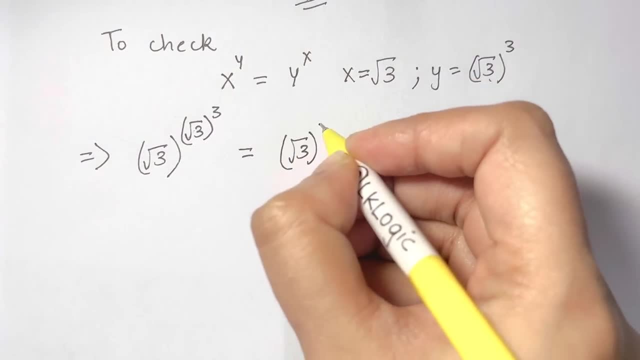 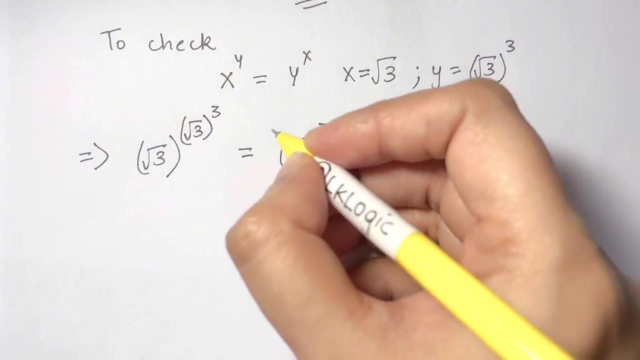 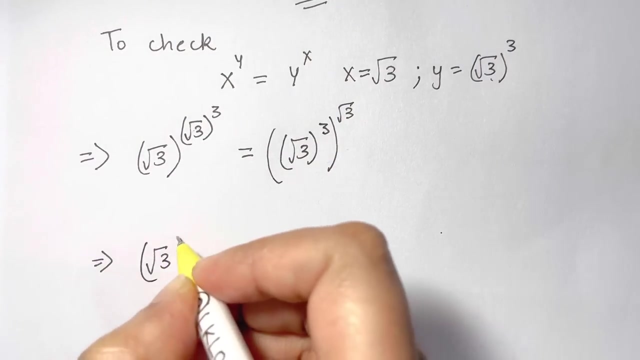 3 whole to the power of 3 over x, and x is root 3. so i have whole to the power of root 3. we have root 3 over this. root 3 can be written as square root, so root always goes into the denominator. so we have 3 to the power of 1 over 2, and this is times 3. 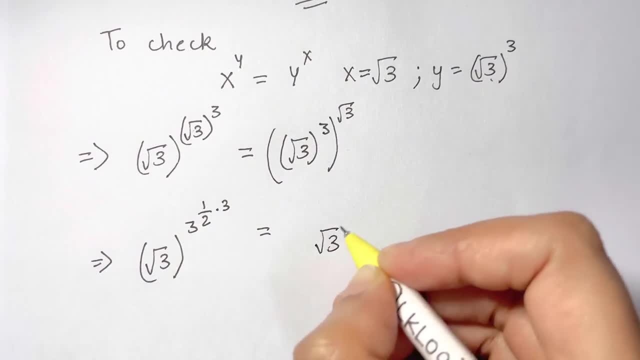 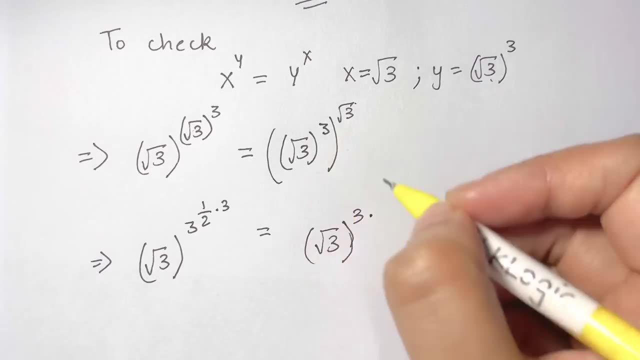 which is equal to 2 square root of 3 over you have 3 and this power to power, you can multiply the powers and square root of 3, root always goes to the denominator. so you have 3 to the power of 1 over 2. now you have: 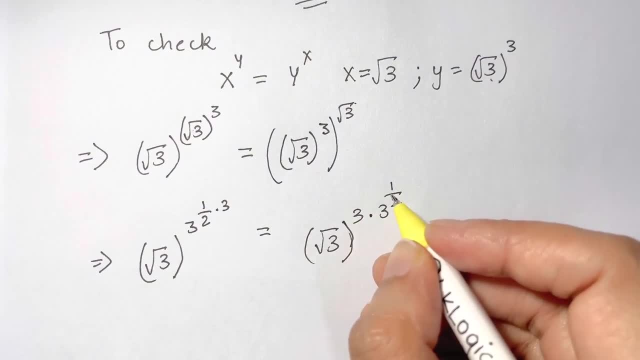 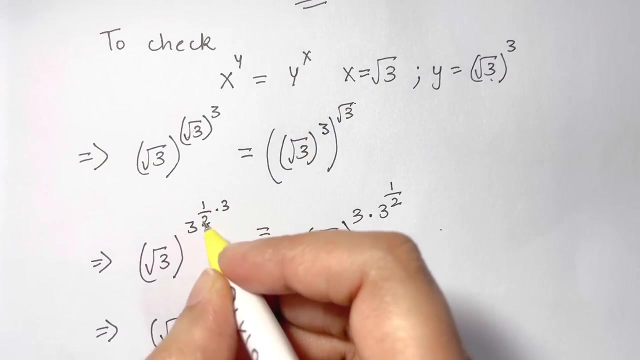 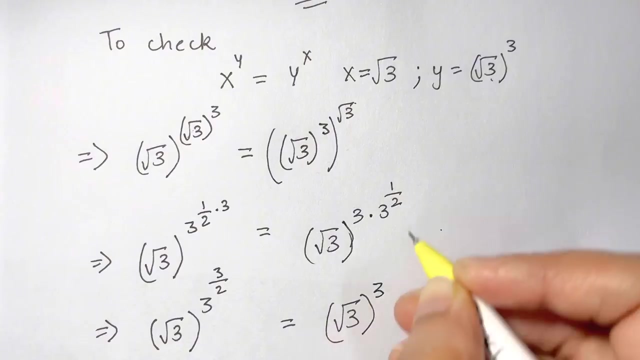 same basis here and there's multiplication, so you can add the powers. so here, what are we going to get is, for this one, square root of 3 whole to the power of 3, to the power of 3 over 2. you multiply the powers here 3 times 1 over 2 and here, square root of 3 whole to the power of 3, and this is you.